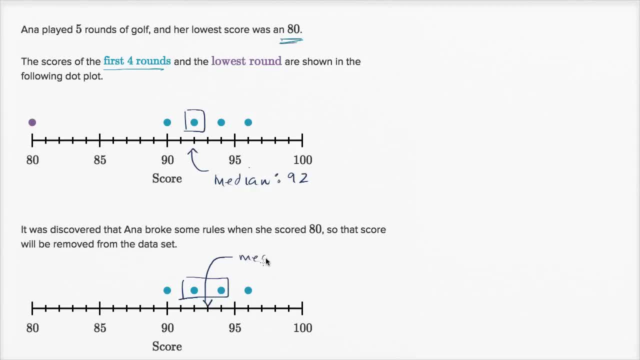 So the median. the median is 93. Median is 93. So removing the lowest data point, in this case, increased the median. So the median let me write it down here. So the median increased by a little bit. The median increases. 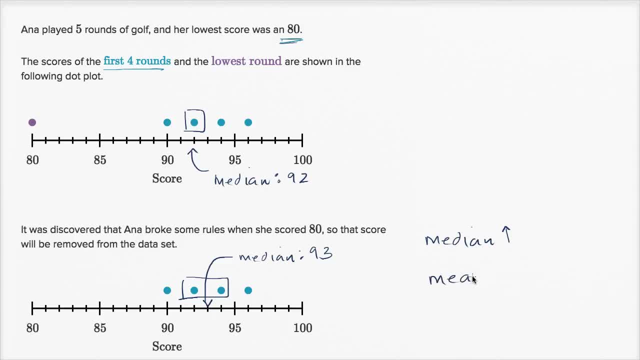 Now, what's going to happen to the mean? What's going to happen to the mean? Well, one way to think about it, without even doing any calculations, is if you remove a number that is lower than the mean, lower than the existing mean. 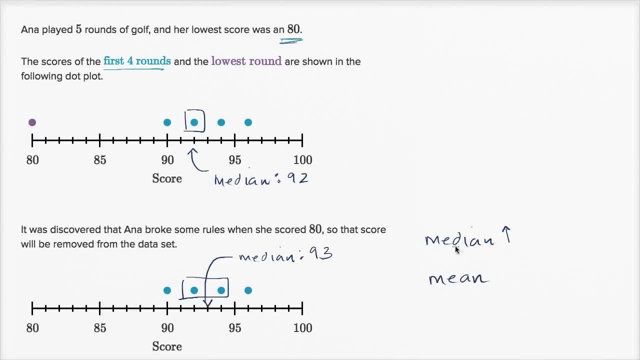 and I haven't calculated what the existing mean is. if you remove that, the mean is going to go up. The mean is going to go up, So hopefully that gives you some intuition If you removed a number that's larger than the mean. 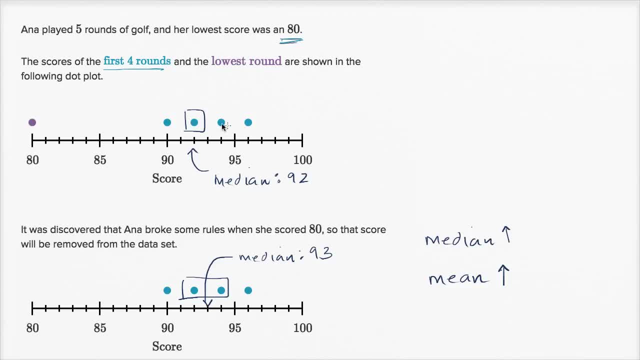 your mean is. your mean is going to go down because you don't have that large number anymore. If you have removed a number that's lower than the mean, well, you take that out. You don't have that small number, bringing the average down. 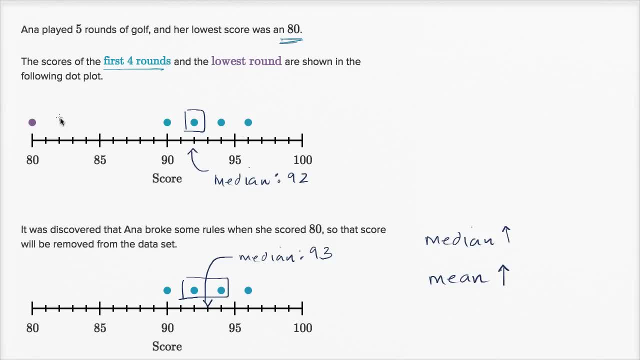 and so the mean will go up. But let's verify it mathematically, So let's calculate the mean over here. So we're gonna add 80 plus 90.. 90 plus 92 plus 94 plus 96.. Those are our data points. 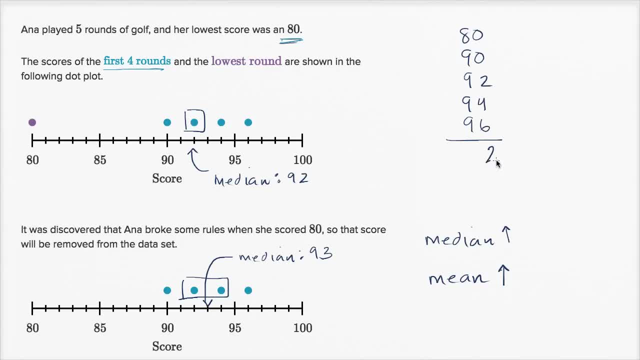 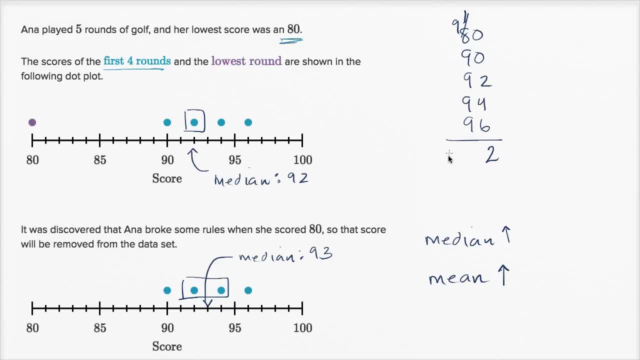 You essentially have. what is this? five, nines right over here. So this is going to be 450, 452.. So that's the sum of the scores of these five rounds, And then you divide it by the number of rounds you have. 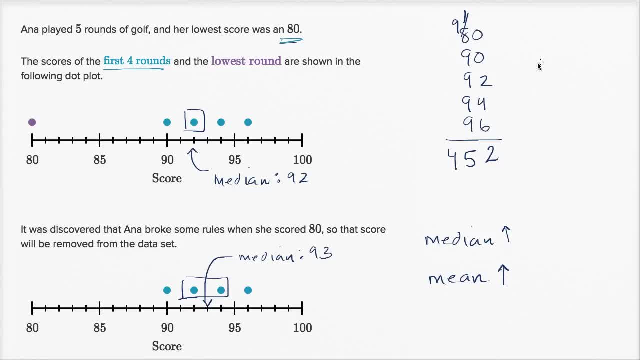 So it would be 452 divided by five. So 452 divided by five is going to give us: five goes into. it doesn't go into four. it goes into 45 nine times. Nine times five is 45.. You subtract. 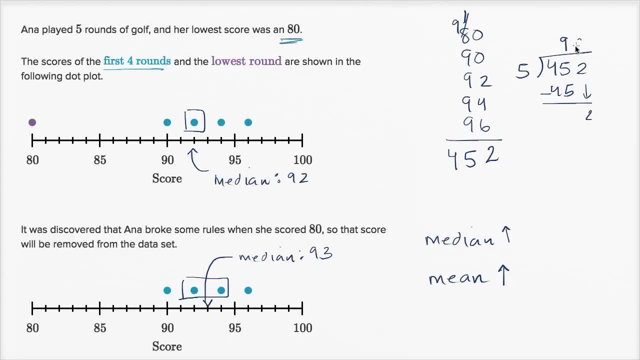 You get zero. bring down the two, Five goes into two is zero times Zero. times five is zero times five is zero subtract, Subtract. you have two left over, So you can say that the mean here, the mean here, is 90 and two-fifths. 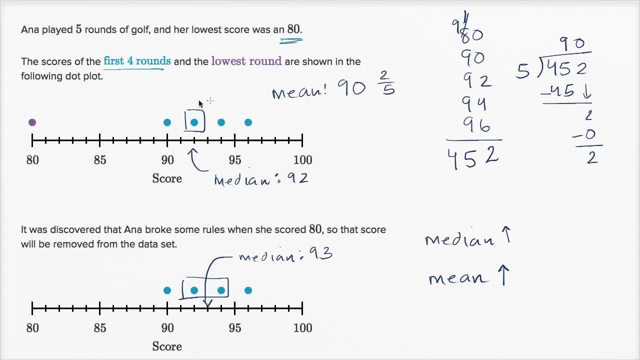 Maybe not nine and two-fifths, 90 and two-fifths. So the mean is right around here. So that's the mean of these data points right over there. And if you remove it, what is the mean going to be? 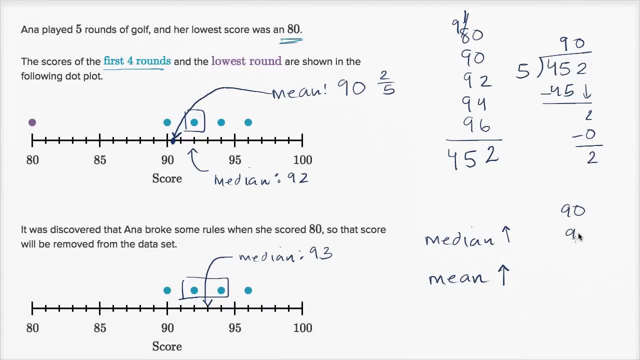 So here we're just gonna take our 90 plus our 92 plus our 94 plus our 96.. Add them together. So let's see: two plus four plus six is 12.. And you add these together you're gonna get 37.. 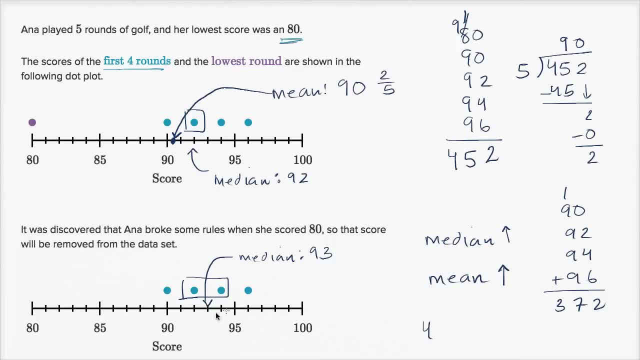 372 divided by four- because I have four data points, now not five- Four goes into three. let me do this in a place where you can see it. So four goes into 372, goes into 37. nine times. Nine times four is 36.. 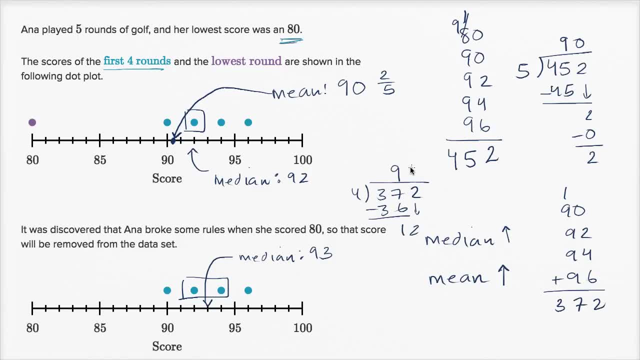 Subtract: get a one, bring down the two, It goes exactly three times. Three times four is 12.. You have no remainder. So the median and the mean here are both. So this is also the mean. The mean here is also 93.. 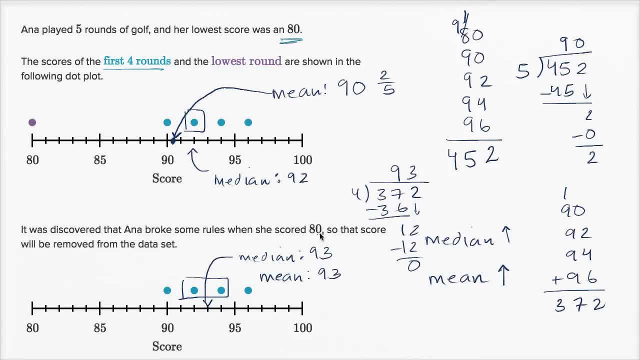 So you see that the median, the median, went from 92 to 93, it increased. The mean went from 90 and two-fifths to 93. So the mean increased by more than the mean. They both increased, but the mean increased by more. 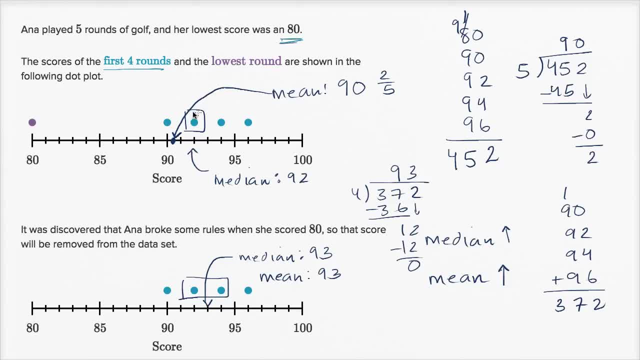 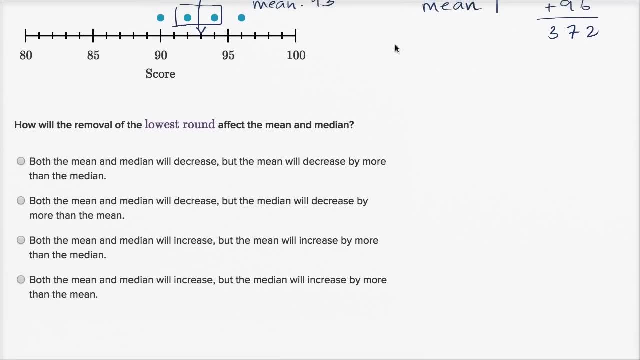 And it makes sense, because this number was way, way below all of these over here. So you can imagine, if you take this out, the mean should increase by a good amount. But let's see which of these choices are what we just described. 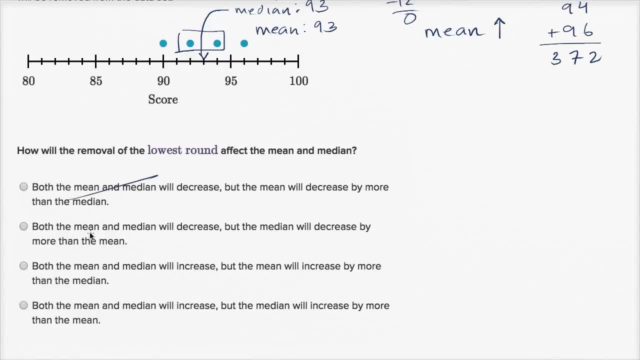 Both the mean and the median will decrease. Nope, Both the mean and the median will decrease. Nope, Both the mean and the median will increase, but the mean will increase by more than the median. That's exactly. that's exactly what happened. 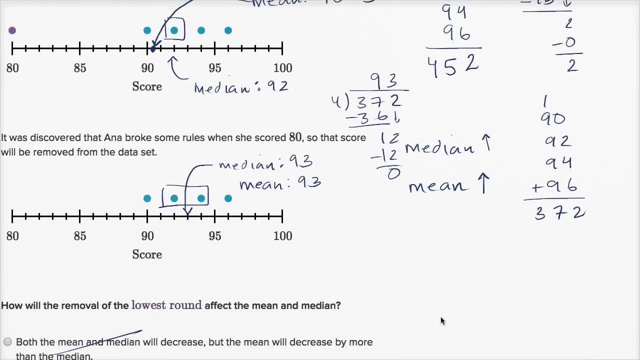 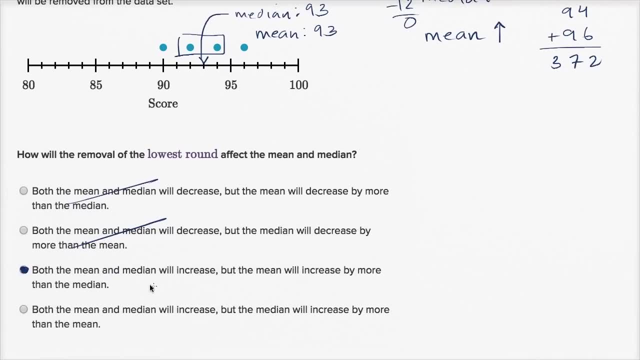 The mean went from 90 and two-fifths or 90.4,, went from 90.4, or 90 and two-fifths to 93, and then the median only increased by one. So this is the right answer.